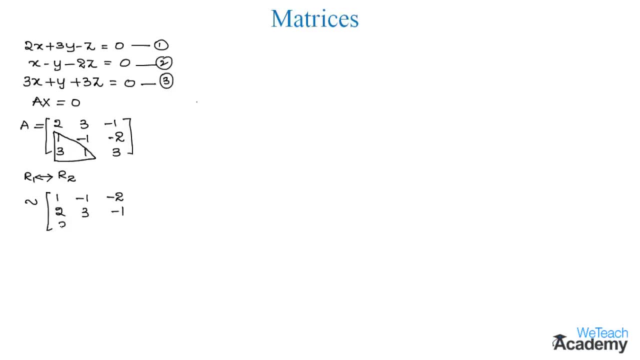 the second row would be 2,, 3 and minus 1, and the last row is 3,, 1 and 3.. And here we need to convert these elements as 0.. So in order to convert the elements 2 as 0, we need to use the transformation of row. 2 implies 2, x R1.. And similarly, to make element 3 as 0, we need to perform the operation. R3 implies 3, x R1.. So in order to use that transformation, we need to calculate the transformation. of row 2 as 0, or R2 minus 2 times of R1, And similarly to make element 3 as 0, we need to perform the operation. R3 implies R3 minus 3x R1, and the same was observed in the first. 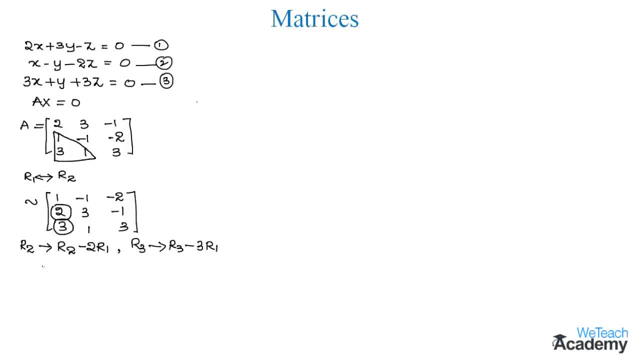 minus 3R1.. So after performing these operations, the matrix E will be similar to the first row: 1 minus 1 minus 2, and in the second row we get here 2 minus 2, which is 0, and then 3 minus of. 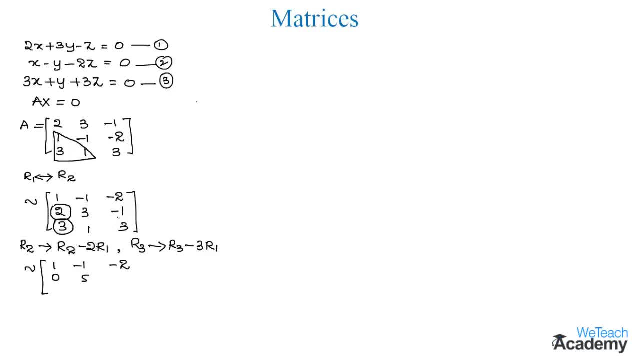 minus 2, which will be 5, and then here, minus 1, minus of minus 2, into 2, which will become minus 1 plus 4.. In turn, we get 3, and now, by performing the operation to row 3, we get 3 minus 3, which is. 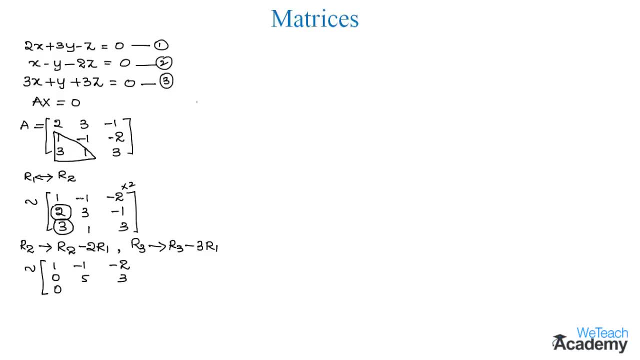 0, then 1 minus of minus 3, which becomes plus 3.. So we get 1 plus 3, that is 4, and then the next element would be 3 minus of minus 6.. So in turn we get 9, and now we need to convert this element. 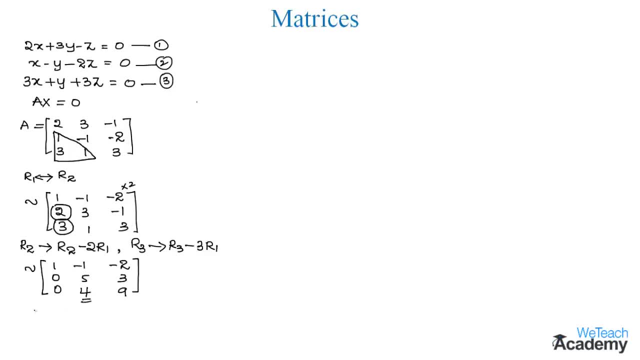 as 0.. So for this we need to make changes. So, in order to make changes to row 3, which is denoted by the notation, So in order to make this element as 0, we can make use of this row and also this row, But as we have the element 0, 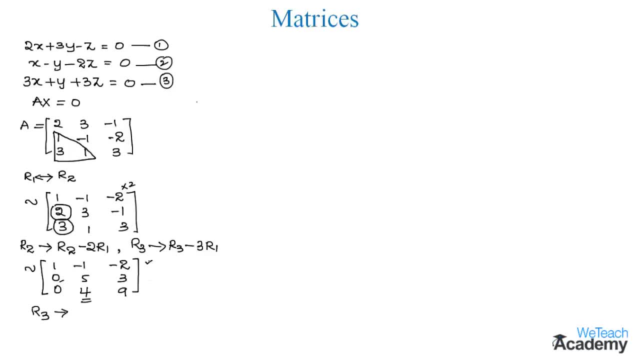 in the second row, we are not going to use R1.. Instead of R1, we are going to use R2.. So by multiplying 5 to R3 minus of, and here by multiplying 4 to R2, we get minus 4R2.. So by performing this, operation, we will get 0.. So, after performing this operation to row 3, we need to make changes to row 3, which is denoted by the notation. So, in order to make this element as 0, we can make use of: 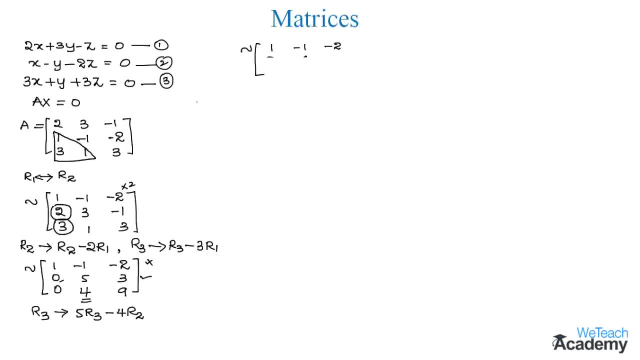 The matrix A will be similar to the first and second row remains the same And the third row will be 0.. Then, using the operation, we get 20 minus 20, that will be 0.. And here, in the last element, we get 9 into 5, which is 45, minus 3 into 4, which is 12.. 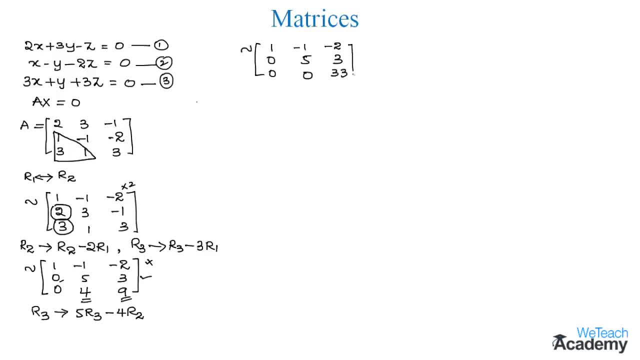 So 45 minus 12 is 33.. And now let us divide the row 3 with 33, which is represented by the notation add 3 implies add 3 divided by 33.. So the matrix A will be similar to 1 minus 1, then minus 2.. 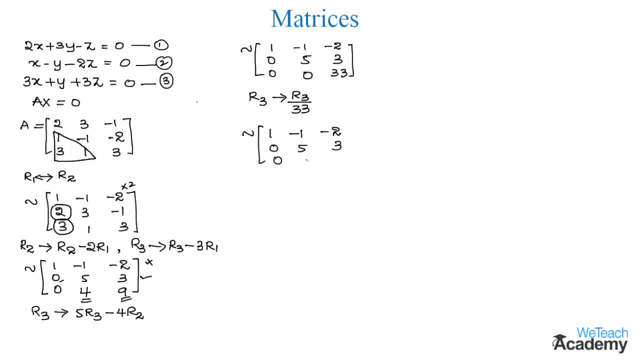 And the next row: 0,, 5,, 3.. And the last row: 0,, 0 and 1.. So now let us name this matrix as equation 4.. And here you can observe that we have converted upper triangular elements as 0.. 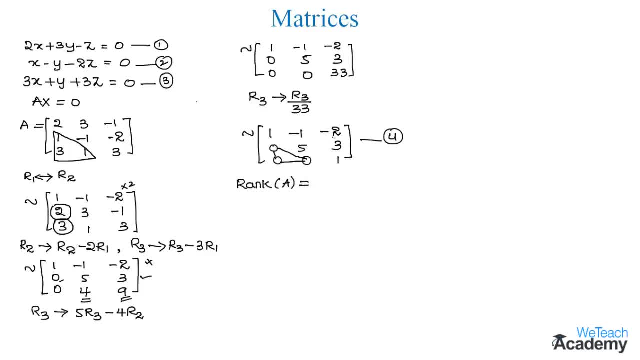 So now we can find the rank of a matrix A, which will be equal to number of non-zero rows. So by observing the columns in equation 4, there are 3 non-zero rows, So hence we can say that the rank of a matrix A is equal to 3.. 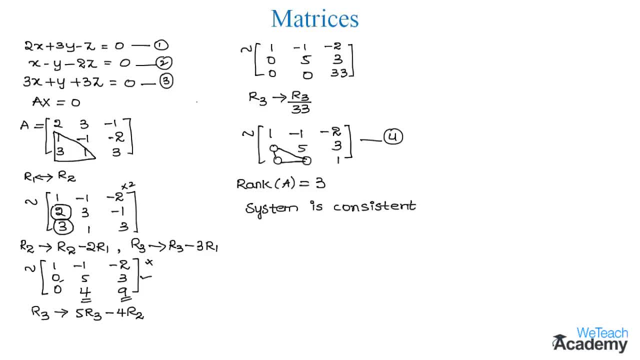 So, therefore, the system of equations is consistent and it has a trivial solution. It means the solutions of these equations will be x equal to y equal to z equal to 0.. Here we already know the solution, So let us check by just finding. 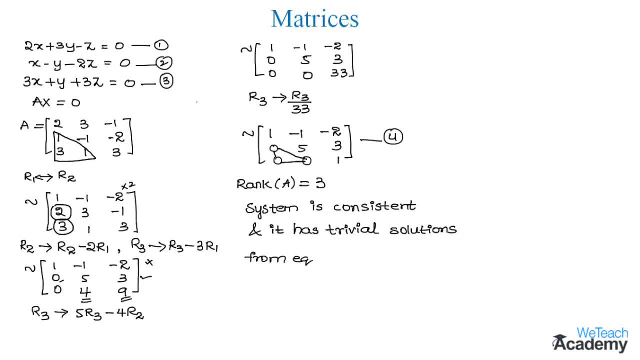 The solutions from equation 4.. So here we get 1 into x, plus of the next element, minus 1 into y, plus of the next element, minus 2 into z is equal to 0.. So from the second row we get 0 into x, plus 5 into y, plus 3 into z is equal to 0.. 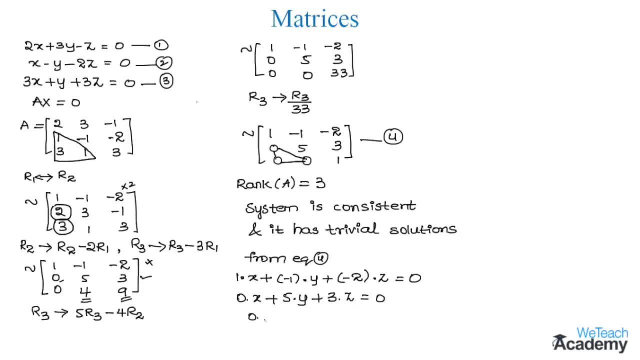 And from the last row we get the equation: 0 into x, plus 0 into y, plus 1 into z is equal to 0.. So now let us name these equations as equation 5, equation 6, and equation 7..